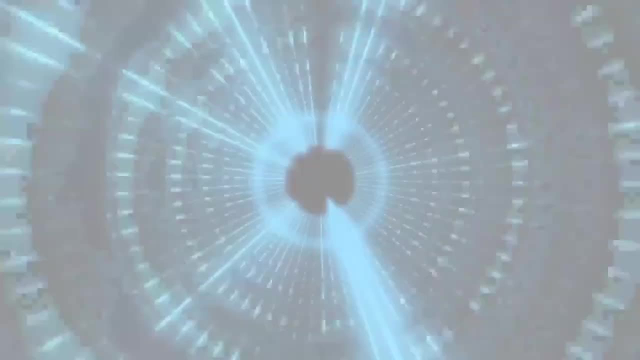 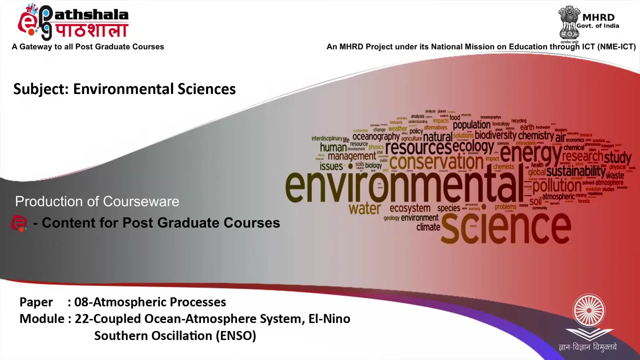 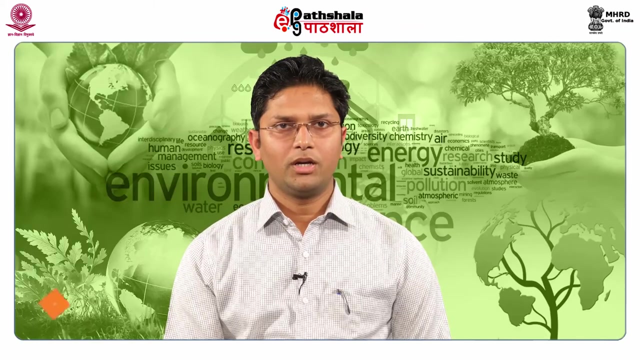 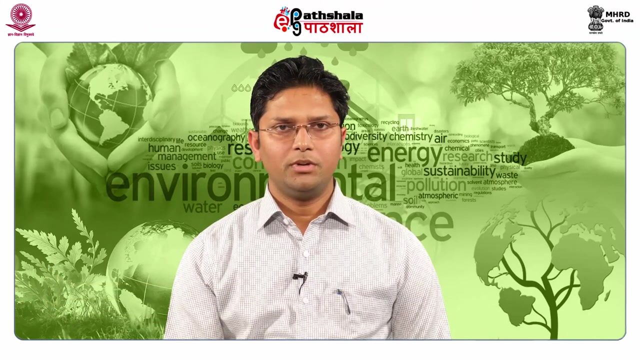 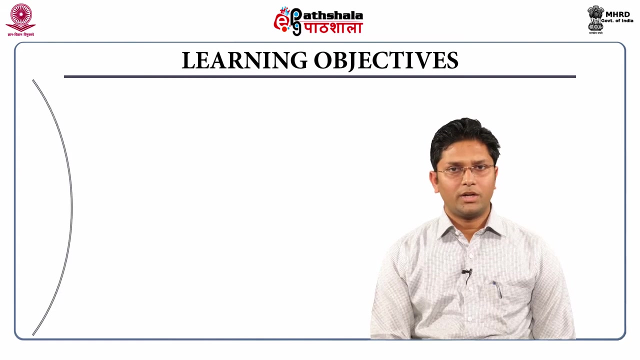 Hello students, welcome to EEPG Parsala. In this session, we shall discuss the topic Coupled Ocean Atmospheric System and El Nino Southern Oscillation. At the end of the presentation, you will be able to answer the following questions: What is a Coupled Ocean Atmospheric System? 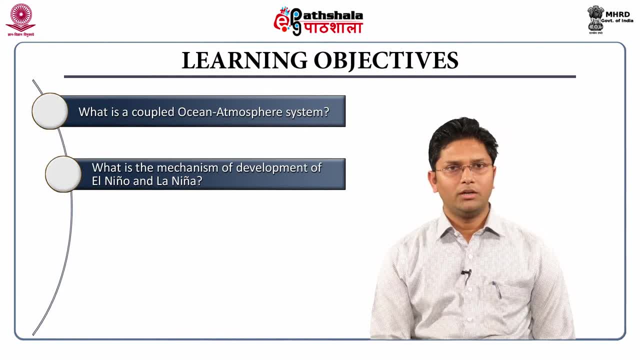 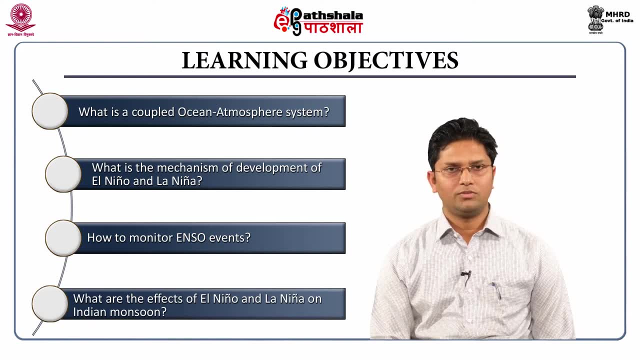 What is the mechanism of development of El Nino and La Nina, How to monitor El Nino Southern Oscillation events And what are the effects of El Nino and La Nina on Indian monsoon? The notion that drought in India, Indonesia and Philippines could be caused by the same. 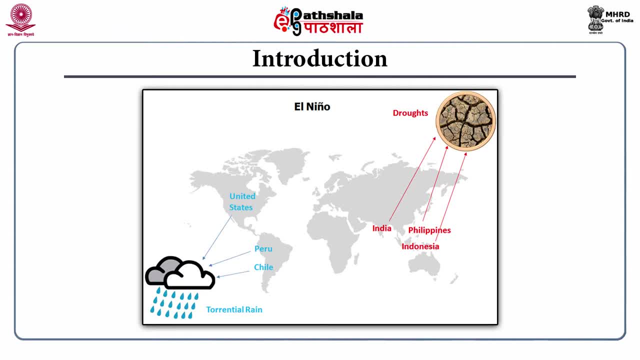 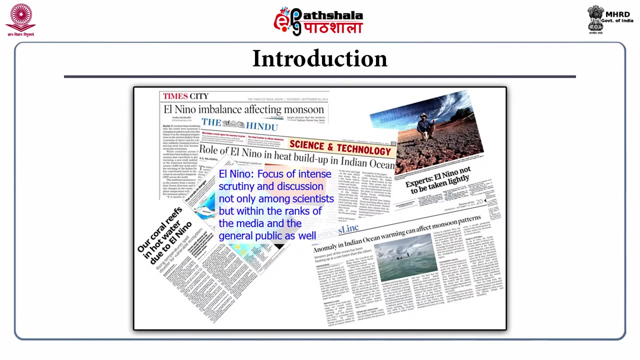 condition that produced torrential rains in the United States, Peru and Chile might appear to the casual observer to defy logic, But in fact that is exactly what can happen during the extraordinary change of events known as El Nino. In the recent years, El Nino events have become the focus of intense discussion, and not only 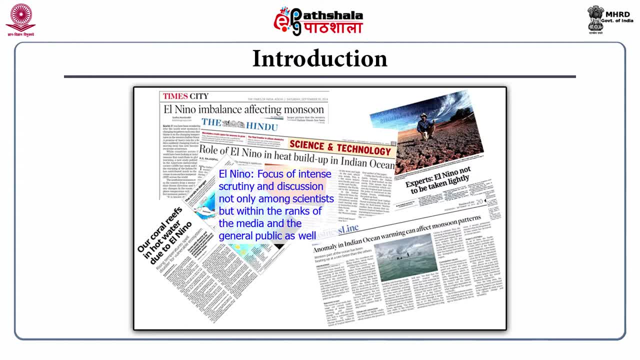 among the scientific community, but also within the ranks of the media and the general public as well. However, the conditions that give rise to these events have been well observed before a century. El Nino and La Nina are the large-scale coupled ocean atmospheric 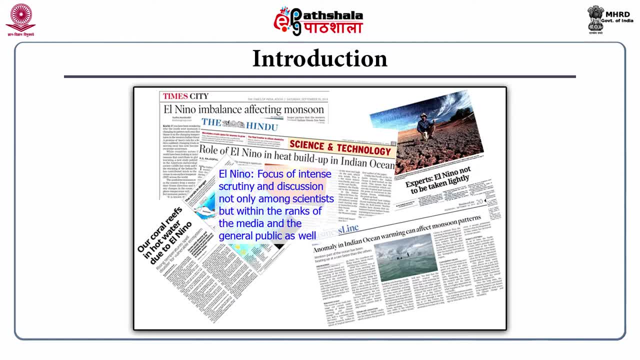 phenomena linked to a period of time in the history of the Indian monsoon season. The two major warming and cooling events are the Earthquake- Equatorial Sandstorm Earthquake and Earthquake El Nino and La Nina are the most important teams of the seven major volcano formations. 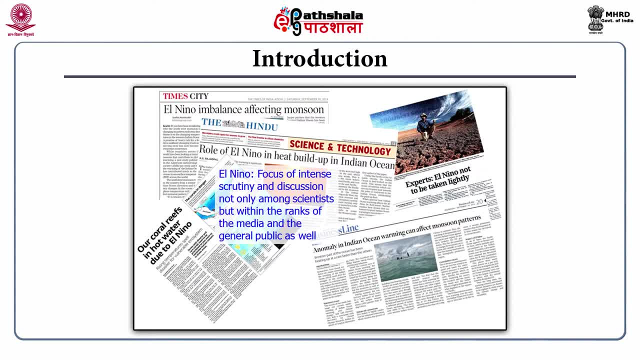 that have been formed to create global warming. The three most important giants: the Theosophic and the Sino-Spanic- five major volcanoes across the central and east-central region of Equatorial Pacific. The genesis behind their formation is very complicated. The five major volcanoes are thought to be the most important because 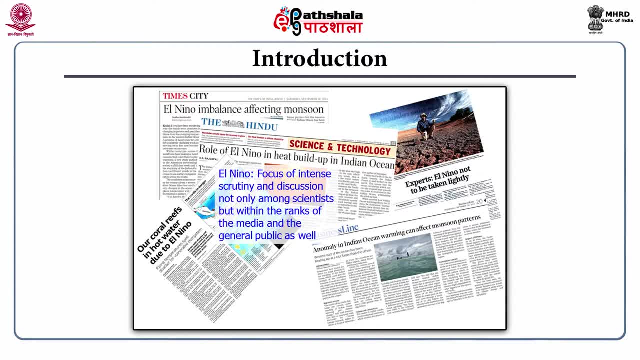 of their global impact. Global impact in the sense they cause drought, flood, increased precipitation, hurricanes or wildfires around different corners of the globe. They also have a direct impact on the global food market or global economy. The Indian Monsoon Rainfall has a highly among the five major volcanoes and is the only one that has been made to. 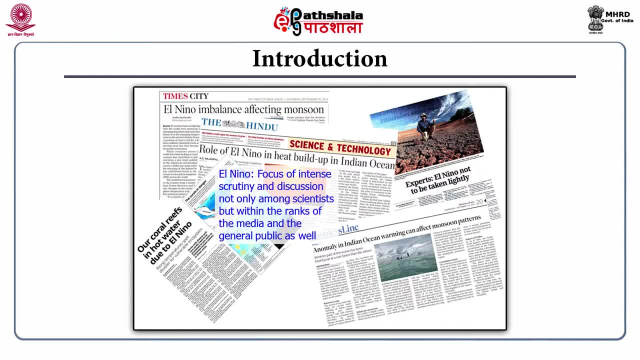 with the global meteorological situations which are technically called as Southern oscillations. Together, El Nino and Southern oscillation are known popularly as NSO. Now let me explain some of the technical terms that I shall be frequently using during this discussion. 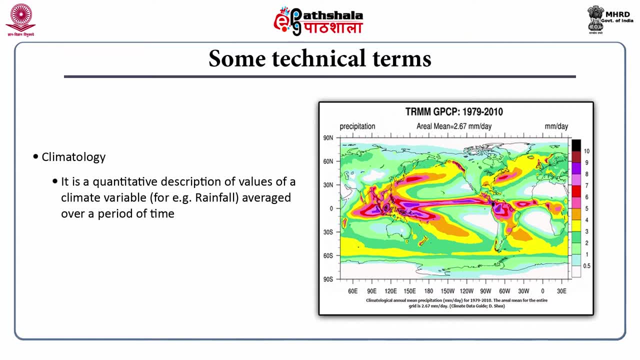 Climatology. it is a quantitative description of values of a climatic variable averaged over a period of time. For example, the case of rainfall has been given here. From this figure we can say that the rainfall over most locations of the oceans are, in general, higher than the landmasses. 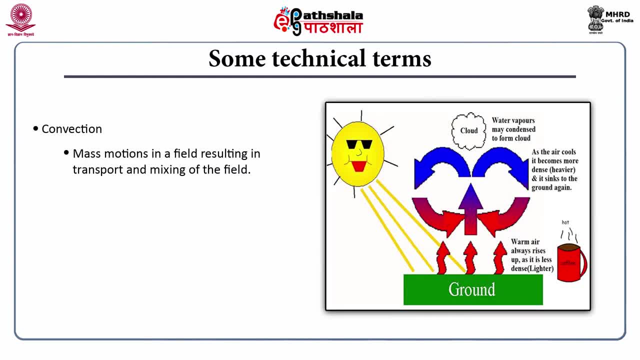 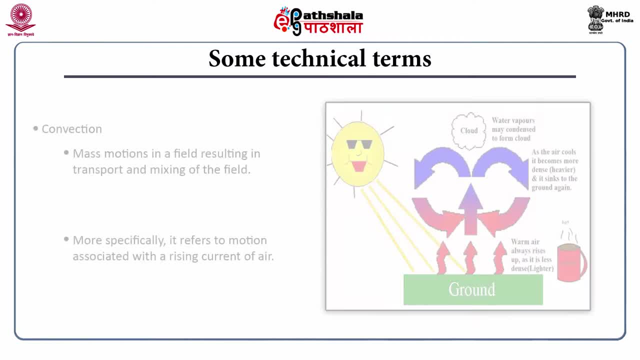 Convection. it is a mass motion in a field, resulting in transport and mixing of the field. More specifically, it refers to motion associated with a rising current of air, Then equatorial upwelling. it is the upward motion of subsurface water toward the surface of the ocean. This is 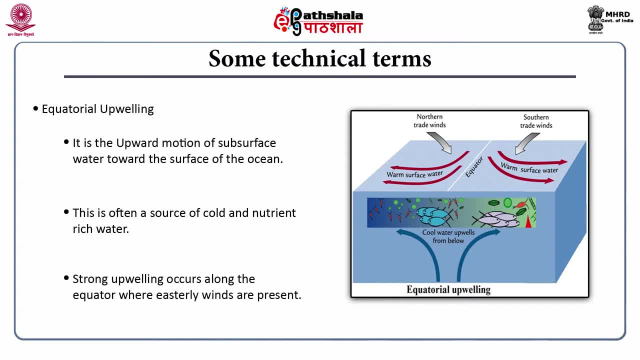 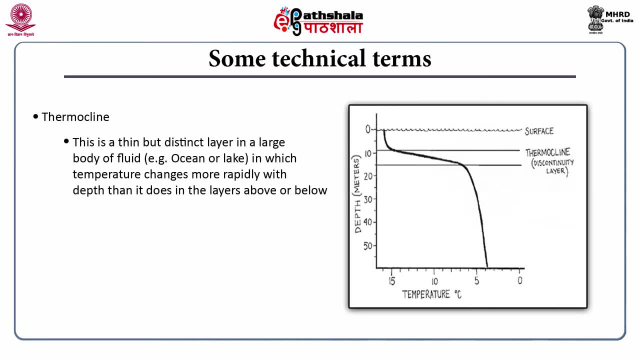 often a source of cold and nutrient-rich water. Strong upwelling occurs along the equator, where easterly winds are present. Thermocline: this is a thin but distinct layer in a large body of fluid like ocean or lake. So in this layer temperature changes more rapidly with depth. 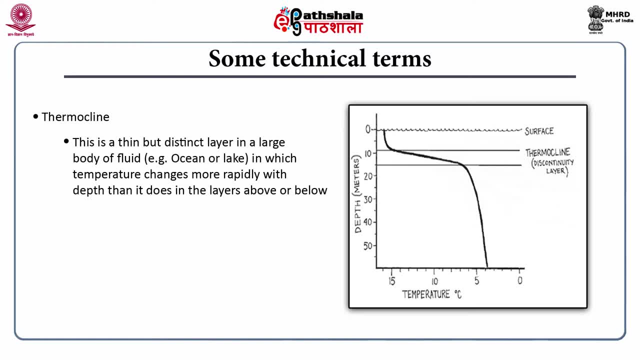 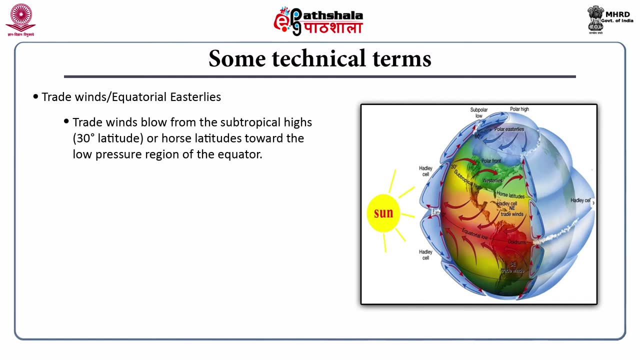 than it does in the layers above or below It forms when water at the surface of an ocean or lake is heated up while the water below that layer stays cool. Now trade winds, or equatorial easterlies. Trade winds blow from the subtropical highs above 30 degrees Celsius. This is a 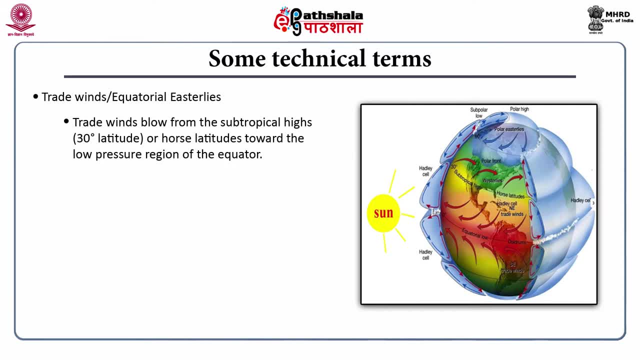 3-degree latitude, or also called horse latitudes. So these winds blow from these subtropical highs towards the low-pressure region of the equator. They are named from their ability to quickly propel trading ships across the ocean In northern hemisphere trade winds. 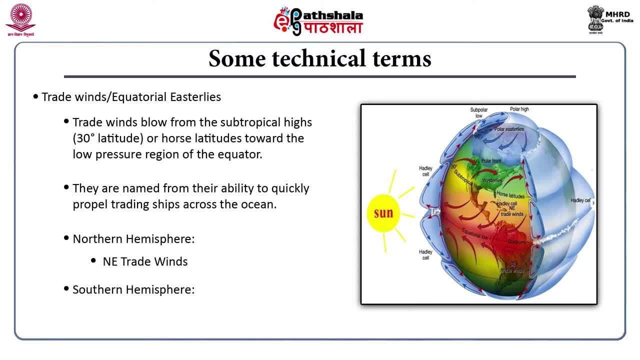 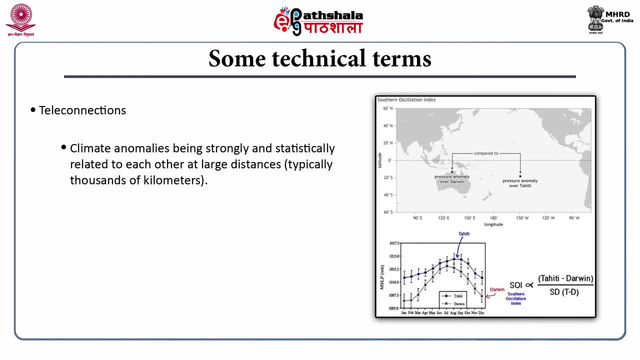 are north-easterly and in southern hemisphere, trade winds are south-easterly, Teleconnections, climate anomalies being strongly and statistically related to each other at large distances, typically thousands of kilometers. Take, for example, linkage of sea level pressure at Tahiti in the Pacific Ocean and Darwin port of Australia. this defines the southern 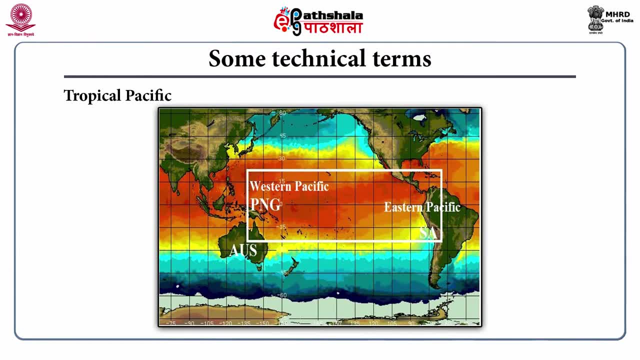 oscillation Now, tropical Pacific. When you mention of tropical Pacific in the NSO context, we are talking about the region marked by red in this figure. In the western part of the tropical Pacific, there is countries like Indonesia, Philippines and Australia, whereas 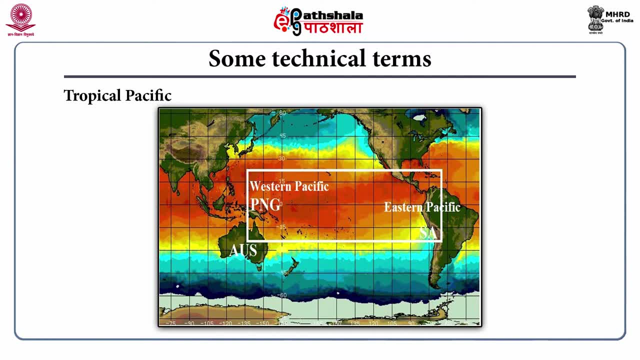 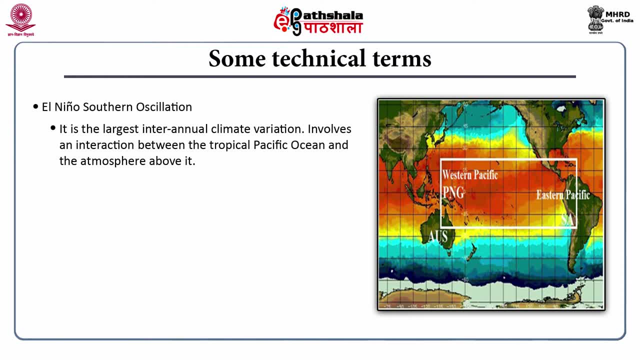 It involves an interaction between the tropical Pacific Ocean and the atmosphere above it. Its impacts are felt worldwide. Heart of the NSO lies in the tropical Pacific Ocean along the equator. Changes in SST, that is, sea surface temperature, ocean subsurface temperature, rainfall and. 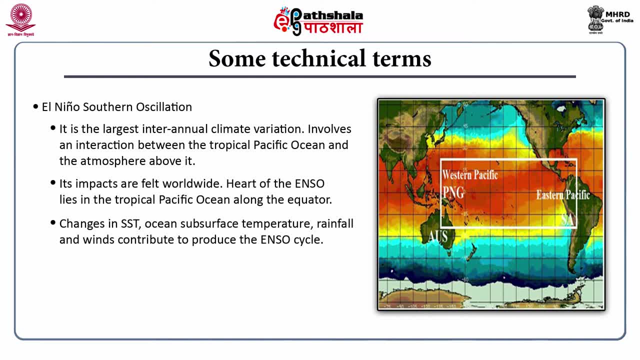 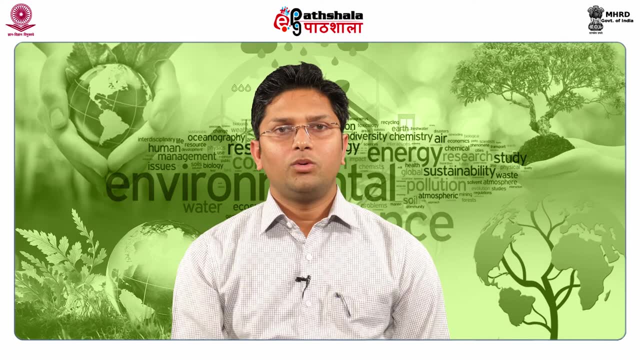 winds contribute to produce the NSO cycle. The variations in the Pacific Basin within about 10 to 15 degree latitude of the equator are the primary variables driving this NSO process. In the few subsequent slides we shall discuss the coupled ocean atmospheric system. 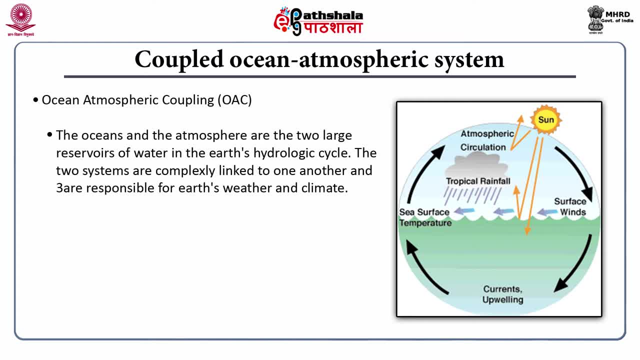 Ocean atmospheric coupling. The oceans and atmosphere are the two large reservoirs of water in the Earth's hydrological cycle. The two systems are complexly linked To one another and are responsible for Earth's weather and climate. Oceans helps to regulate temperature in the lower part of the atmosphere, while the atmosphere 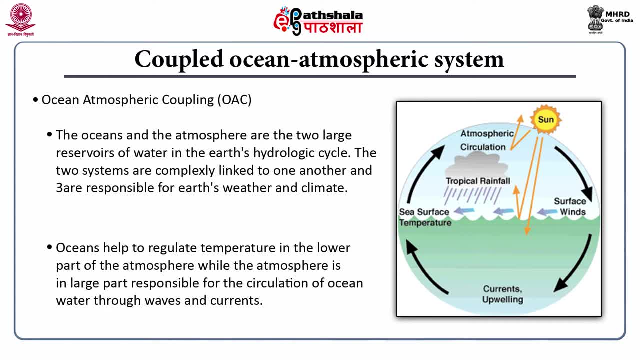 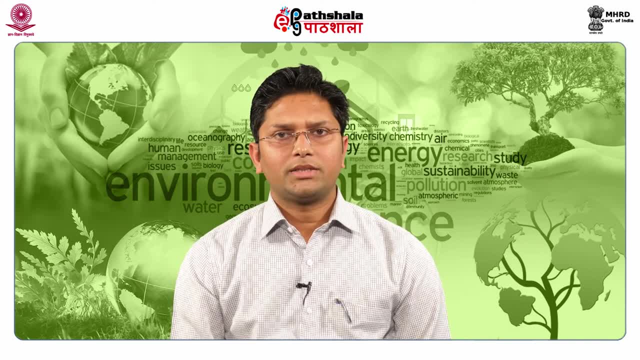 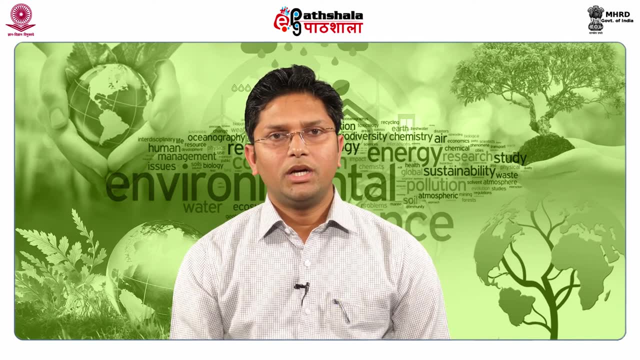 in large part responsible for the circulation of ocean waters through waves and currents. Now let me tell you the theory behind the ocean. atmospheric coupling, A large scale anomaly of sea surface temperature, induces diabetic heating or cooling of the atmosphere, which changes atmospheric circulation and hence the wind stress. 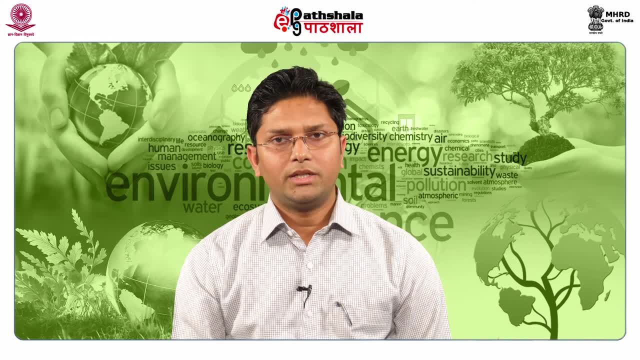 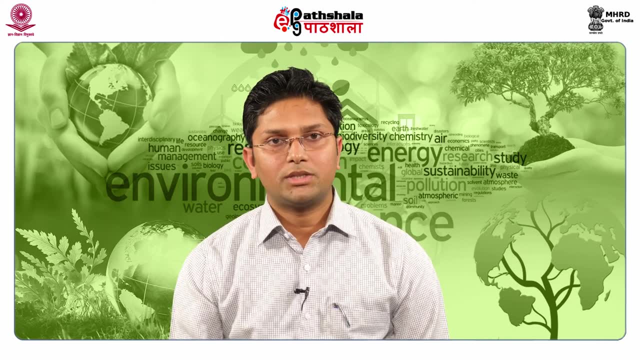 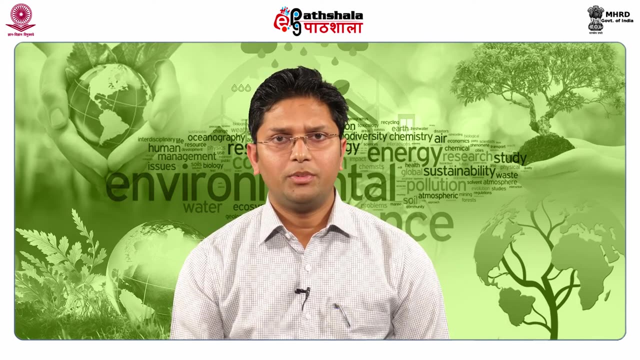 And heat fluxes at the ocean surface. As a result, ocean thermal structure and circulation gets modified, giving rise to a series of positive feedbacks that strengthen the initial SST anomaly. Ocean and atmospheric circulations are interdependent on each other, And the SST serves as a link combining these two elements. 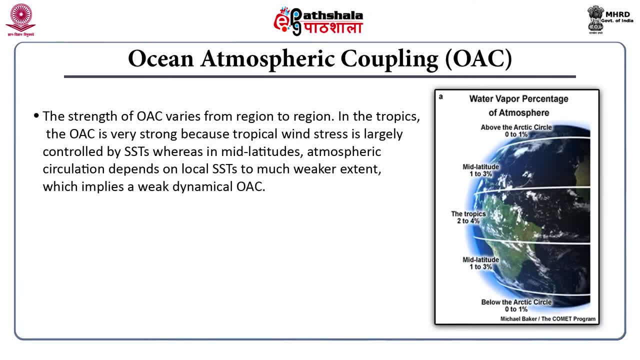 The strength of ocean and atmospheric coupling varies from region to region. In the tropics the coupling is very strong because tropical wind stress is largely controlled by sea surface temperature, whereas in middle latitudes atmospheric circulation depends on local SSTs and the dependence is weaker. 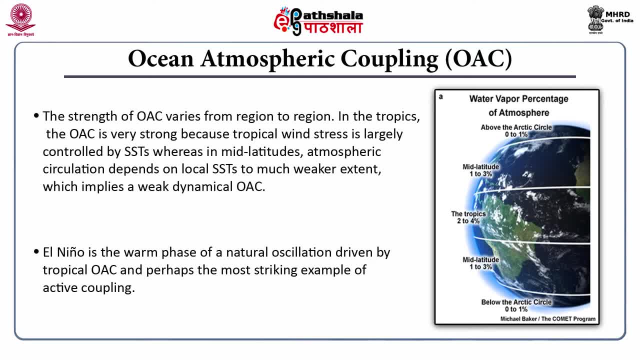 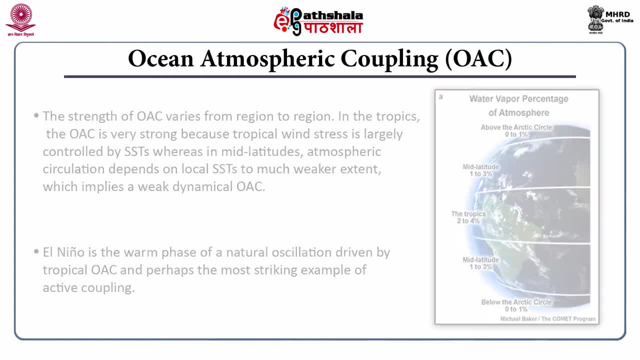 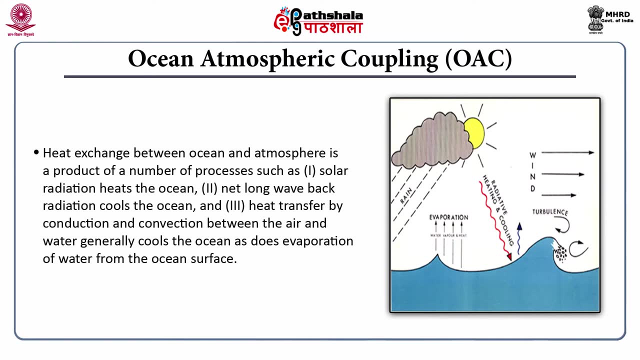 So Illinois is the warm phase of a natural oscillation driven by tropical ocean atmospheric coupling, And perhaps this is the most striking example of active coupling. The exchange between ocean and atmosphere is a product of a number of processes such as solar radiation heats the ocean. 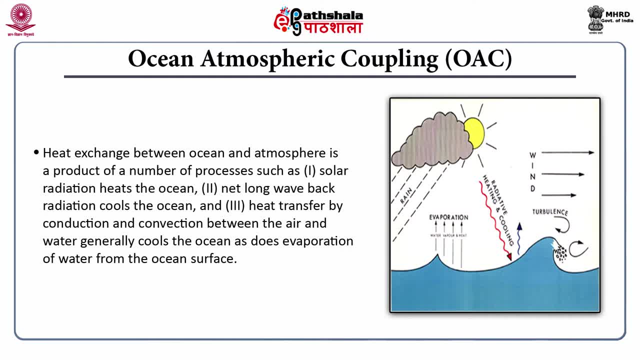 Then ocean radiates back long wave radiation. This process cools the ocean. Then heat is transferred from the ocean to the atmosphere by way of conduction and convection. Also, there is evaporation from the ocean surface, And this evaporation process cools the ocean. 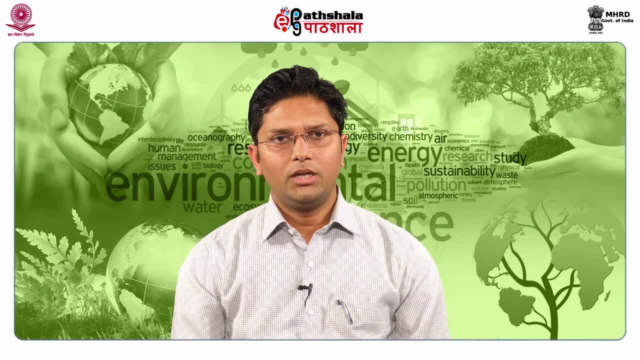 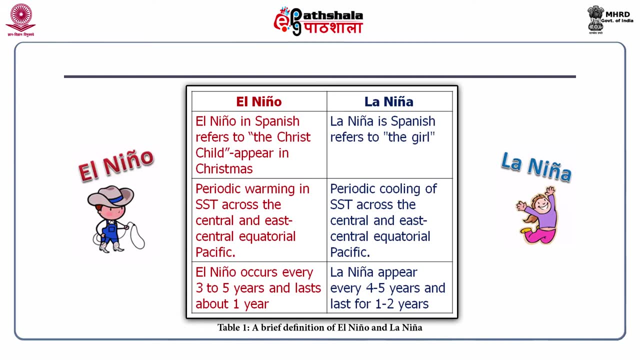 In the few subsequent slides, we shall elaborately discuss about El Nino and La Nina. This topic is now over, Thank you. This table gives a brief definition of El Nino and La Nina. El Nino and La Nina are Spanish words. 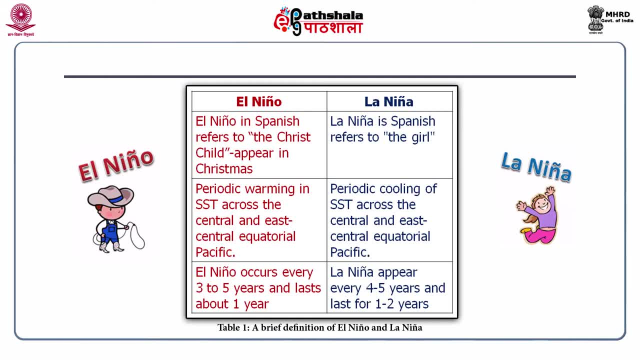 El Nino means the Christ child which appears in the Christmas, And La Nina is the girl child. In case of El Nino, there is periodic warming in the sea surface temperature across the central and east central equatorial Pacific. In case of La Nina, instead of warming, there is a periodic cooling in the same region. El Nino occurs every 3 to 5 years and lasts about 1 year. La Nina appears every 4 to 5 years and lasts for 1 to 2 years. The mechanism and development of El Nino and La Nina. First, let us see how pressure plays a role in it. 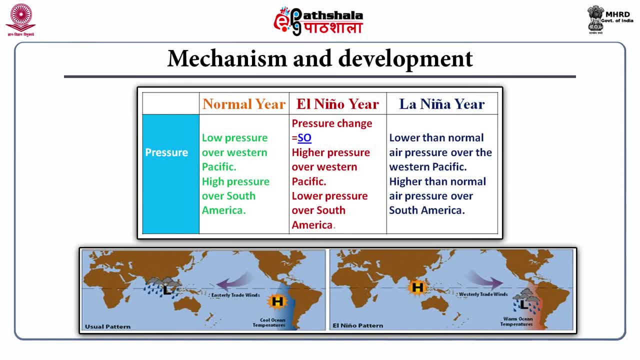 In case of normal air, there is low pressure over Western Pacific region and high pressure over Eastern Pacific region, that is, South American region. In case of La Nina, this pressure changes And this is called Southern Oscillation, That is, during El Nino air. 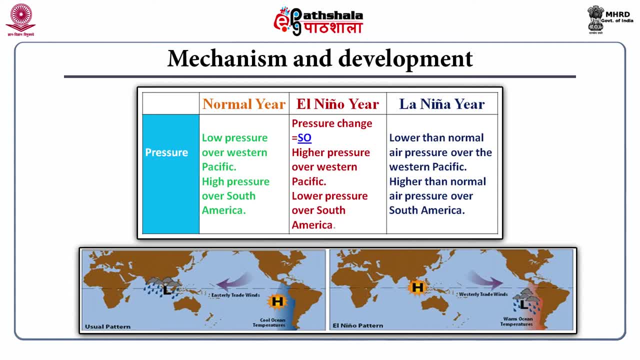 You will find higher pressure, And then this is called Southern Oscillation. That is, during El Nino air You will find higher pressure. That is Southern Oscillation. That is Southern Oscillation over western pacific region and lower pressure over south American region. 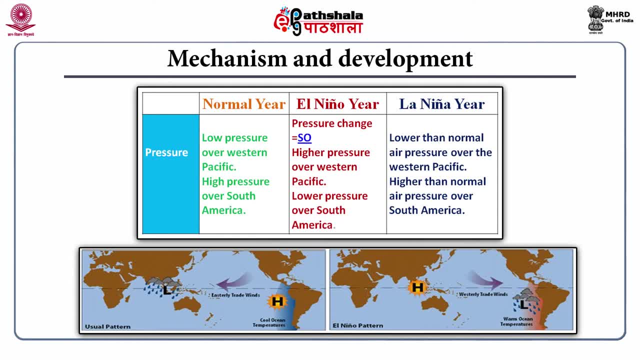 In case of La Nina air, it will be normal air, but the magnitude will be higher, That is, the air pressure over the western pacific will be lower than its normal and the pressure over the south America will be higher than the normal value. 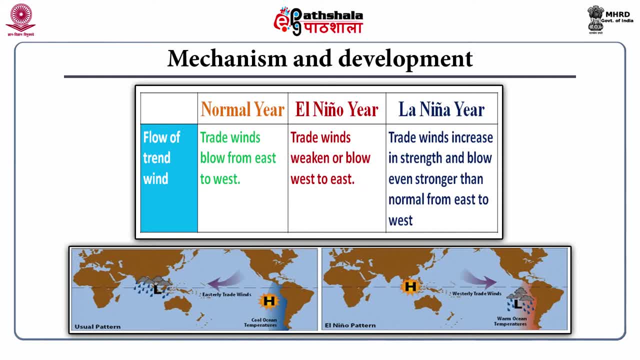 Then flow of trade wind. In normal air, trade winds blow from east to west in the equatorial pacific region, That is, the wind blows from south American side to the Indian Ocean sides and along the wind the ocean water also moves towards the western pacific region. 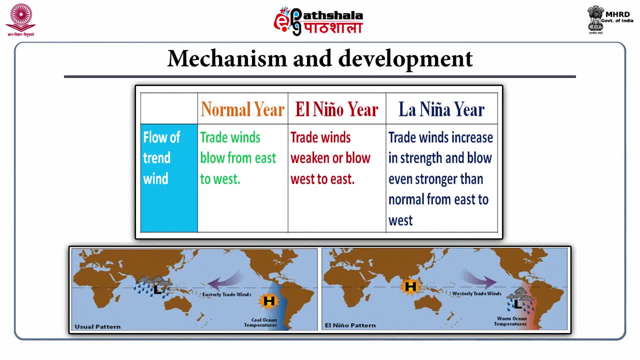 That is why, in a normal air, we will find a higher sea level in the western pacific region than that of eastern pacific region. During a El Nino air trade, winds either weaken or blow from west to east. In case of La Nina air, the winds are steadily only, but the magnitude or strength is higher. 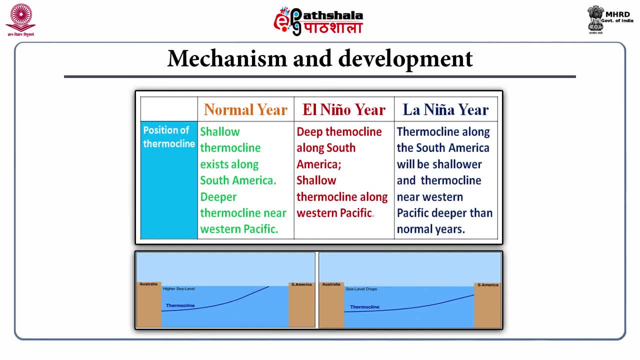 The position of thermocline In a normal air. there exists a shallow thermocline along south America coast and deeper thermocline near the western pacific region. In a El Nino air, the thermocline in the south American side gets deeper and the western 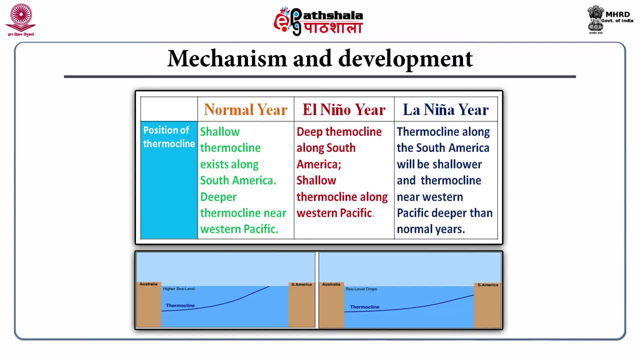 pacific side gets slower. In case of La Nina, air thermocline along the south America will be shallow And thermocline near western pacific is deeper than the normal airs Now upwelling. In a normal air there is a lots of upwelling. 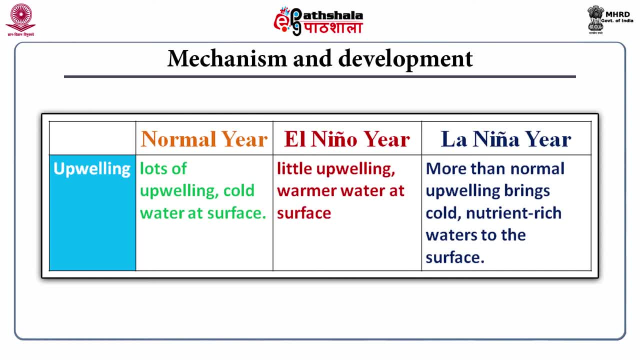 That is, moving of cold water from the underneath of the ocean to the surface, And this upwelling happens off the coast of south America, That is, the eastern pacific region. In case of El Nino air, there will be either little upwelling or no upwelling. 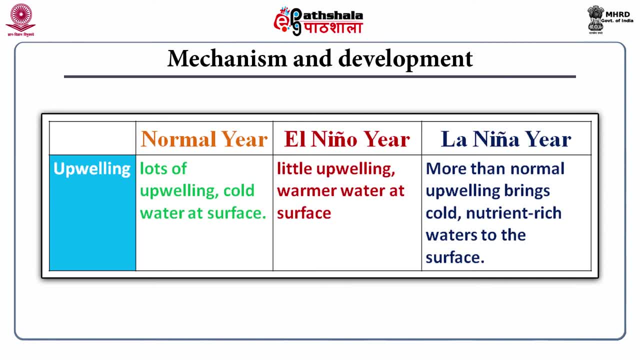 And the water at the ocean surface will be warmer. In case of La Nina air, there will be either little upwelling or no upwelling, And the water at the ocean surface will be warmer. For La Nina air, the upwelling of the Peru coast or the eastern pacific region will be. 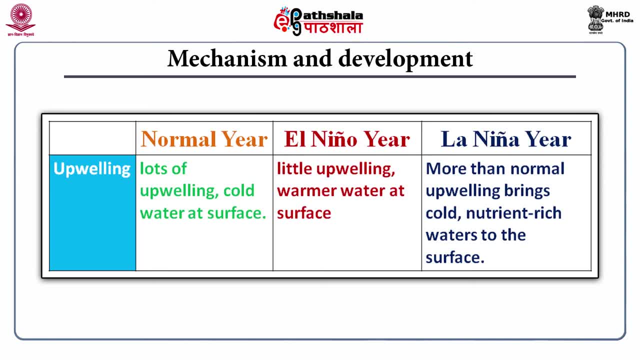 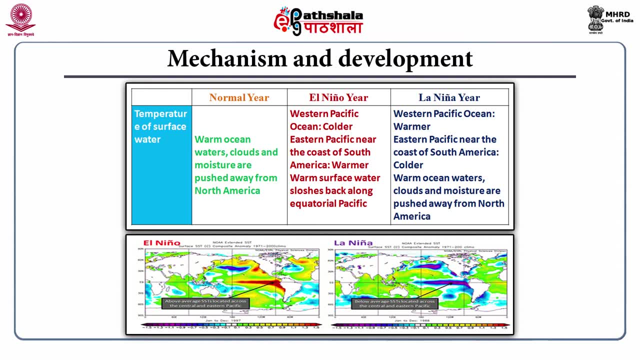 more than the normal, And this upwelling brings cold, nutrient rich water to the surface. Now let us see what role temperature plays in this El Nino, La Nina development. In normal air, warm ocean water, clouds and moisture are pushed away from north American. 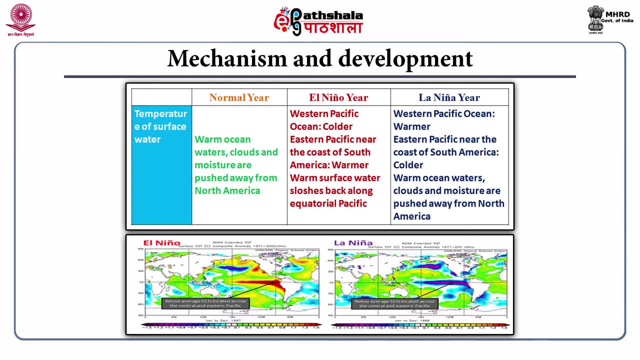 side. In El Nino air, western pacific ocean is colder and eastern pacific near the coast of south America remains warmer. The warm surface water slows back along the equatorial pacific In a La Nina air. western pacific ocean remains warmer, whereas eastern pacific near the coast. 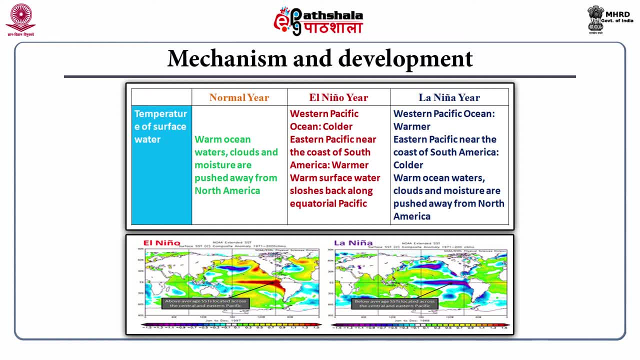 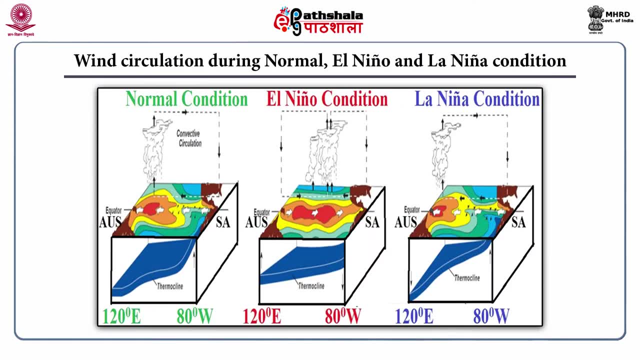 of south America is colder. Warm ocean waters, clouds and moisture are pushed away from the north American side. This figure shows the wind circulation pattern both at the surface level and at higher altitude during normal El Nino and La Nina years, And this is in the atmosphere over tropical pacific. 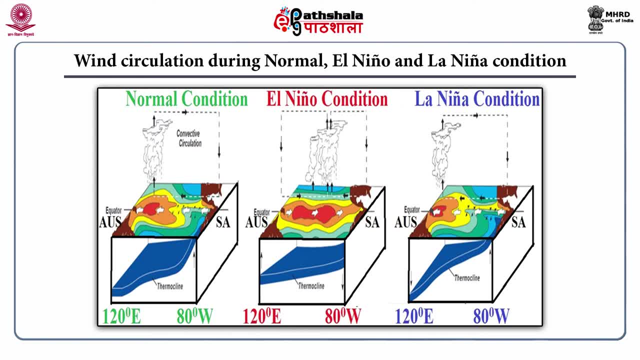 And this figure shows the wind circulation pattern both at the surface level and at higher altitude during normal El Nino and La Nina years, And the region bounded by 120 kms, and this is in the atmosphere over tropical pacific- 120 degree east longitude and 80 degree west longitude. 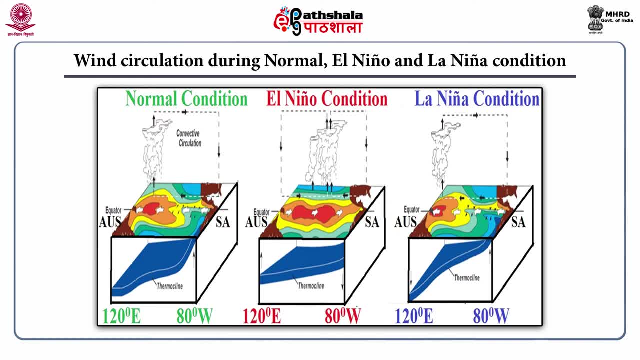 The associated changes in ocean current, then shape of the thermocline and zones of strong convective precipitations are also depicted here. Like in a normal condition, in a normal year, the convective precipitations are generally in the western pacific region, in a land years that ships far of the western pacific and 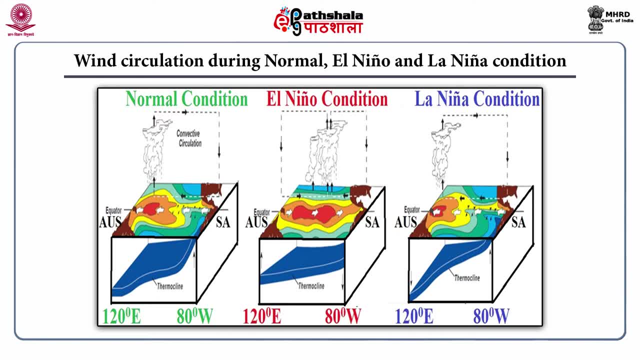 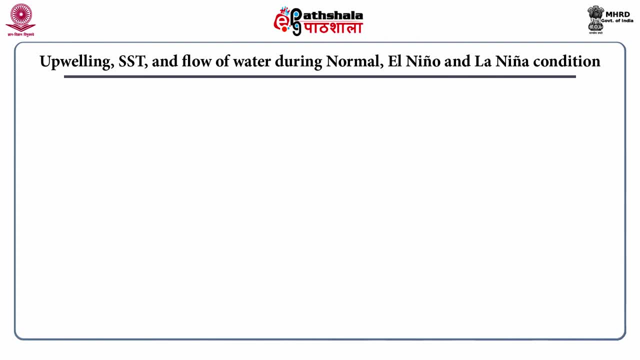 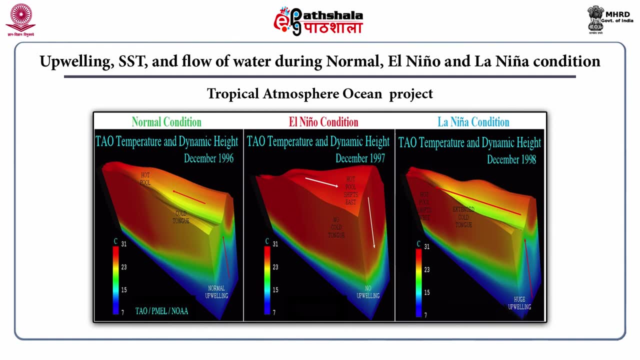 in case of El Nino year, either it is in the central pacific region or towards the eastern pacific region. Upwelling, sea surface temperature and flow of water during normal El Nino and La Nina conditions. These figures have been taken from the reports of tropical ocean atmospheric project. 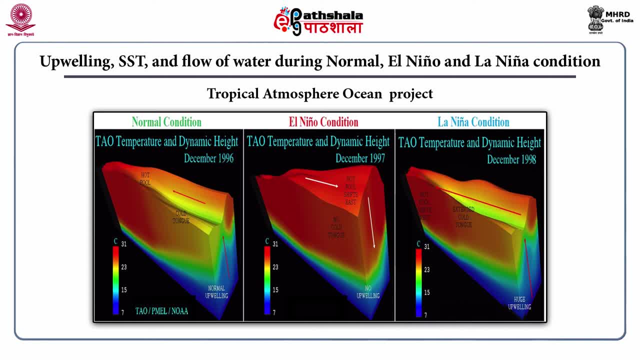 During a normal year the surface height is more in the western pacific sea surface temperature is higher and there is upwelling of cold water near the south American coast, that is, in the eastern pacific region. During El Nino year overall, tropical pacific is warmer, sea level and temperature is higher. 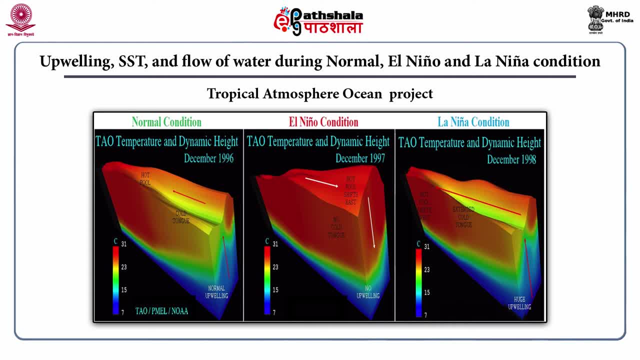 in the southern pacific region During La Nina year. overall, the ocean is cooler than normal, western pacific is warmer and there is a huge upwelling of the Peru coast. that is huge upwelling in the eastern pacific region. 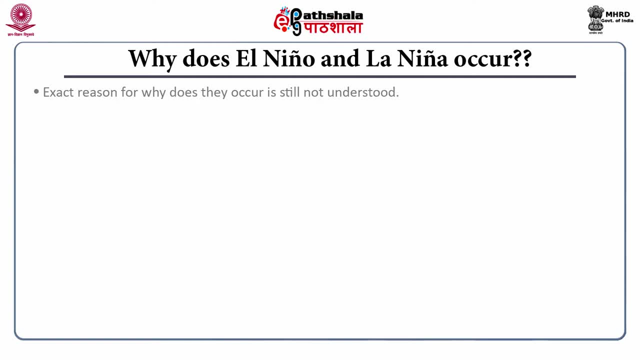 Let us look at the reason. why does El Nino and La Nina occur? Exact reason for why does they occur is still not understood. El Nino results from interaction between the surface layers of the ocean and the overlying atmosphere in the tropical pacific region. 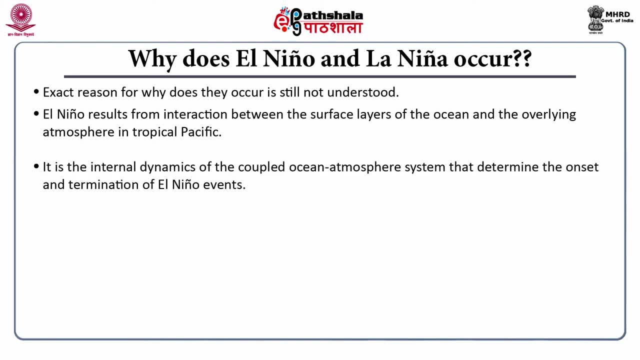 It is the surface layer of the ocean. It is the internal dynamics of the coupled ocean atmospheric system that determine the onset and termination of El Nino. The physical processes are complicated, but they involve unstable air-sea interaction and planetary scale oceanic wave. 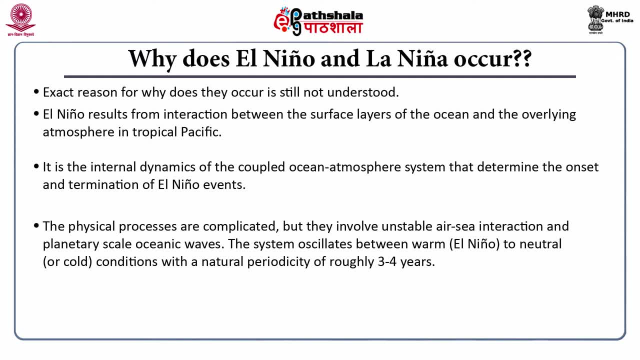 The system oscillates between warm- warm phase, that is, El Nino phase, to neutral or cold phase, that is La Nina phase, with a natural periodicity of roughly about three to four years. External forcing from volcanic eruptions have no connection to the surface layers of the 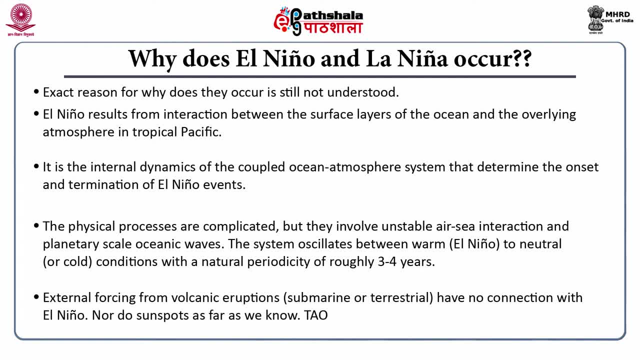 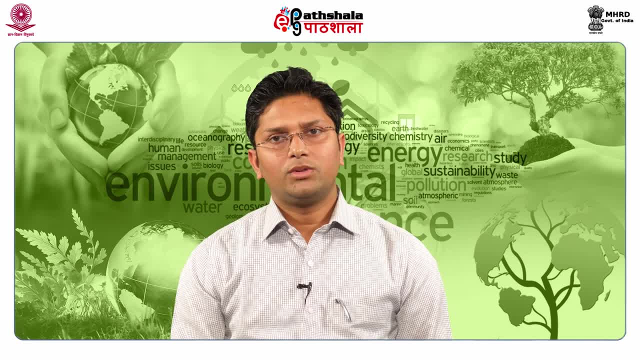 ocean. Also, as far as we know, there is no role of sunspots in bringing El Nino or La Nina. In the next slide we shall discuss how NSO, that is, El Nino and southern oscillation events, are monitored. 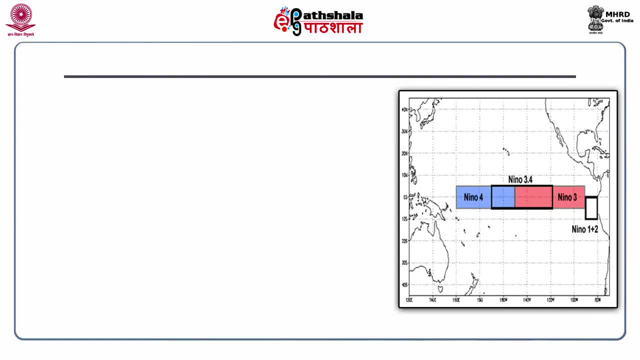 These El Nino and La Nina events are monitored with the help of some indices. These are like Nino 1 plus 2, Nino 3, Nino 3.4 and Nino 4.. Like in case of Nino 1 plus 2.. 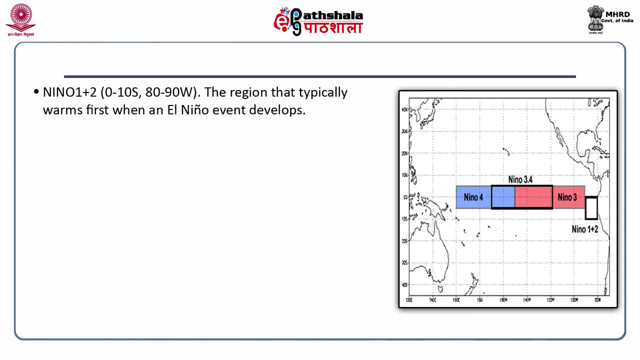 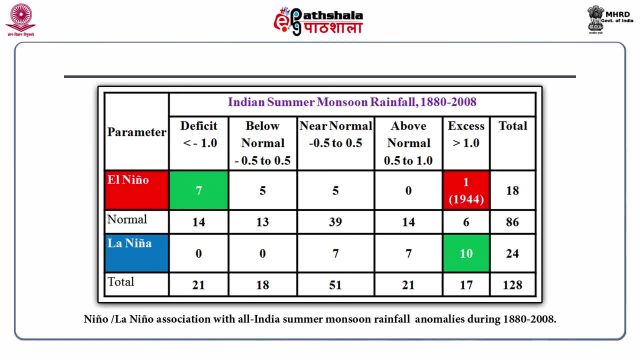 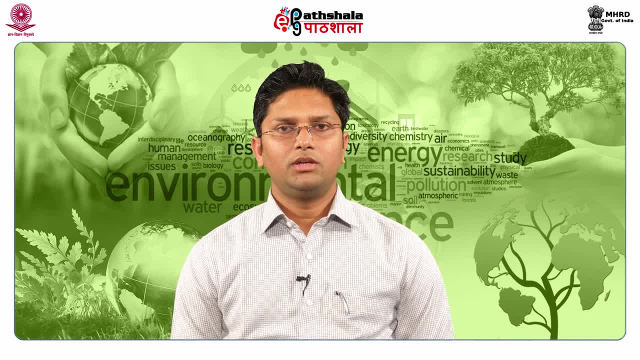 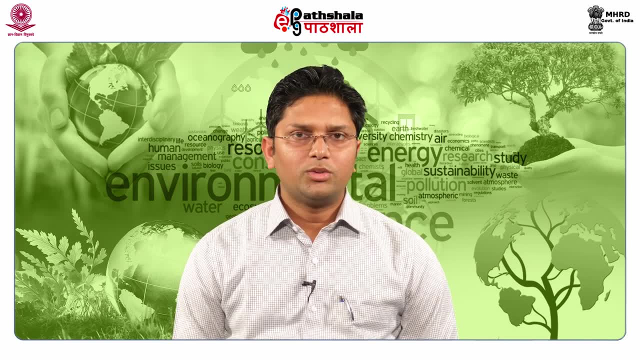 in a years, but only in 10 years. rainfall was excess as per this index. To summarize, the coupling between ocean and atmosphere is straight forward. A large scale anomaly of SST induces diabetic heating or cooling of the atmosphere, which modifies atmospheric circulation as well as the wind stress and heat fluxes at the ocean. 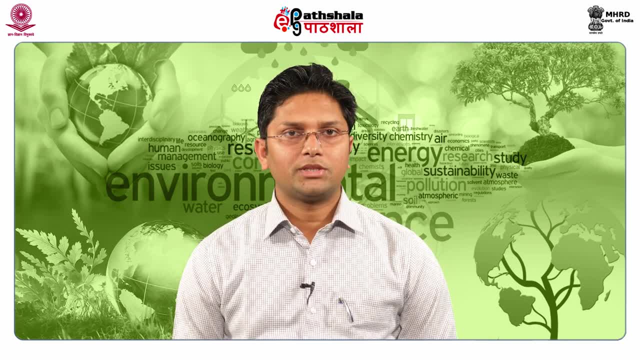 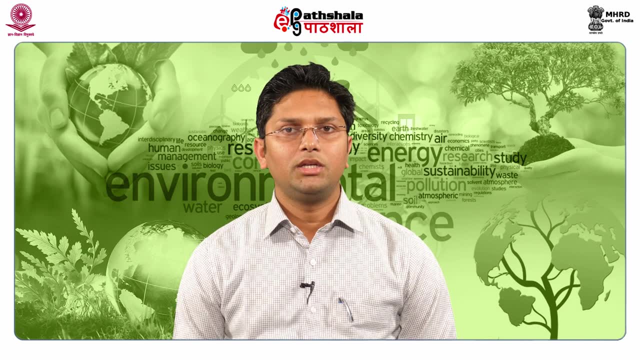 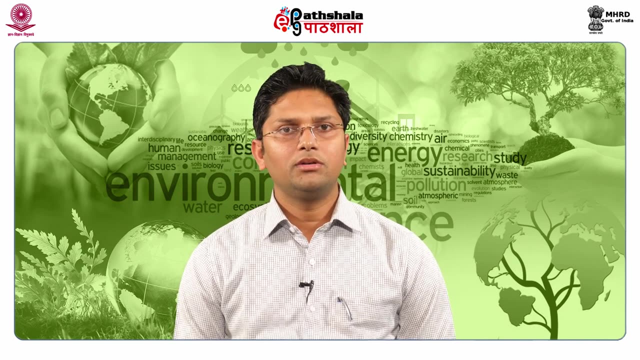 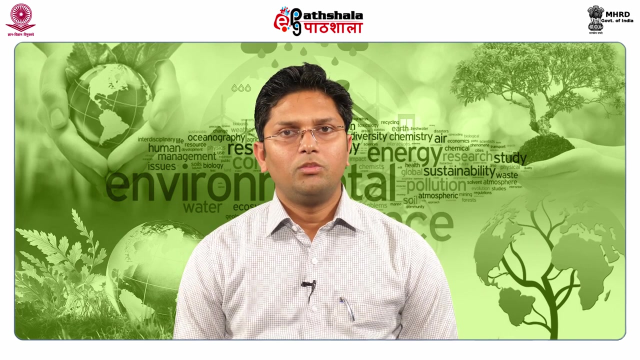 surface. As a result, ocean thermal structure and circulation gets modified, giving rise to a series of positive feedbacks that strengthen the initial SST anomaly. El Nino and La Nina both develop due to large scale interaction of ocean and atmosphere. SST and sea surface pressure are the main drivers of these processes. Both of them have significant impact on a global scale. due to teleconnection, The impacts of El Nino and La Nina are more devastating than the Fortuna. El Nino episode is characterized by deficient or less than normal rainfall in Indian subcontinent, while La Nina episode is characterized by more than normal rainfall in the Indian subcontinent.